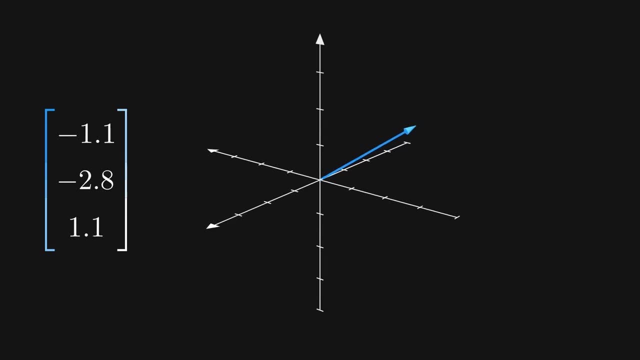 arrow or a vector that goes from the origin to the point instead. and when we do this, it becomes clear that our list of three numbers correspond to combining our unit x, y and z vectors tip to tail. You can write any vector as a combination of these unit x, y and z vectors. They're special. 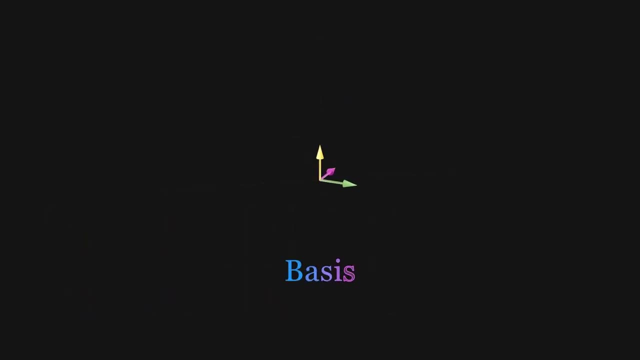 and that's why we call them a basis. They're very important and that's why diagonalization is all about changing the basis. While a column of numbers represents an arrow in space, a square matrix of numbers typically represents what we call a linear transformation. It's a function that takes in vectors and outputs different ones. 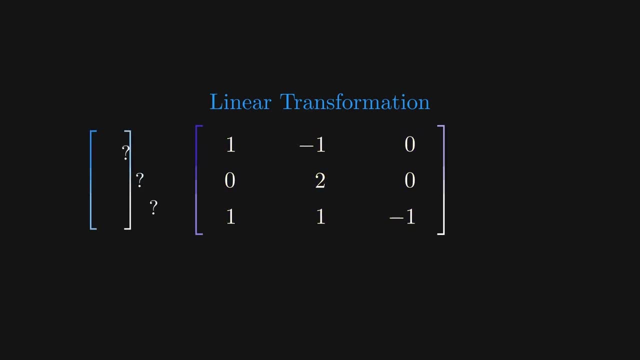 You can calculate this function by scaling each column vector in the matrix and summing row by row to get the output. We can see how this works in practice in 3D. Say we want to input the vector 1, 1, 2 to our transformation. 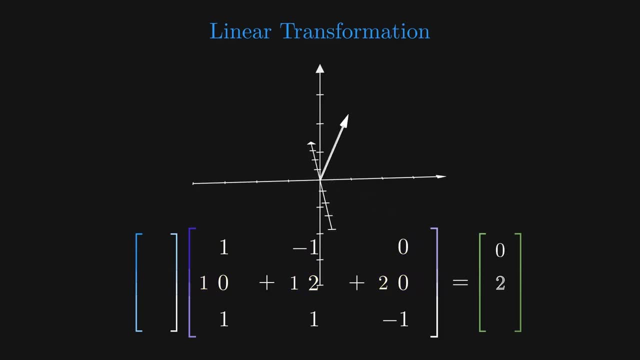 Scaling and summing each row, we see we get the vector 0, 2, 0. So our transformation takes 1, 1, 2 to 0, 2, 0.. If we want to know where our unit x, y and z vectors go, all we have to do 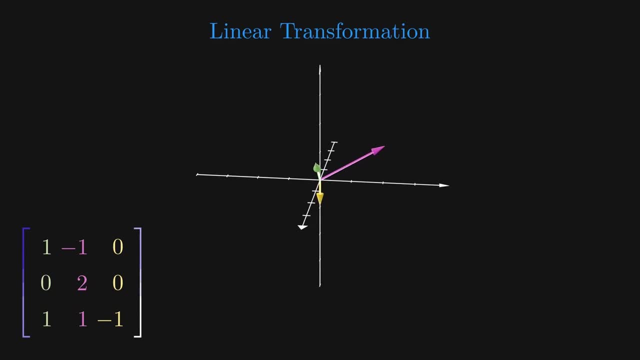 is read off in order: the columns of our matrix. Now, if we know how to transform our unit x, y and z vectors under the transformation, we should be able to transform every point in 3D space with this transformation. And that is exactly what a linear transformation is. It is a 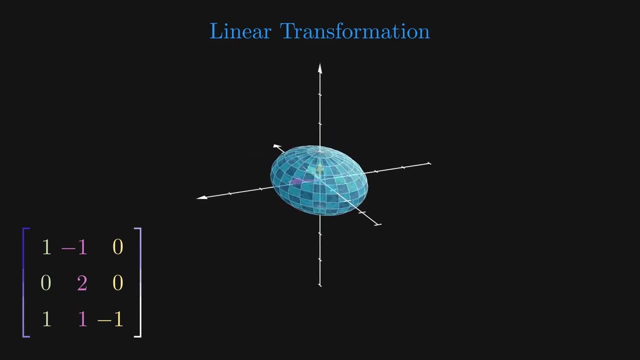 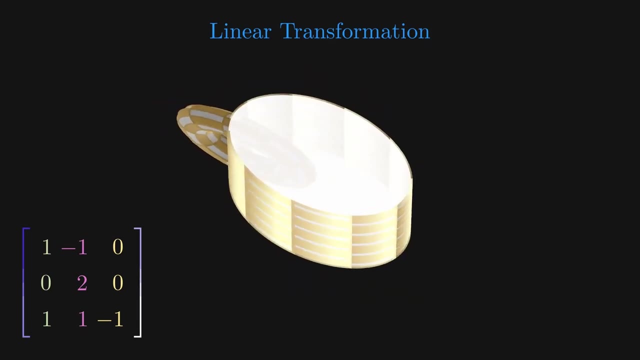 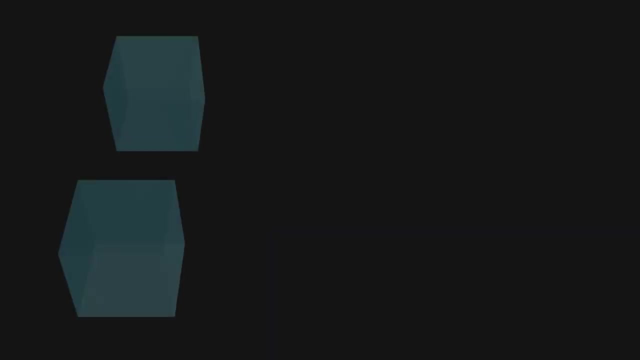 bending or morphing of 3D space. Now, if this is a lot to take in, don't feel bad. The point is that a square matrix of three numbers corresponds to a transformation of 3D space. The tricky thing about linear transformations is that the same transformation of 3D space could have different 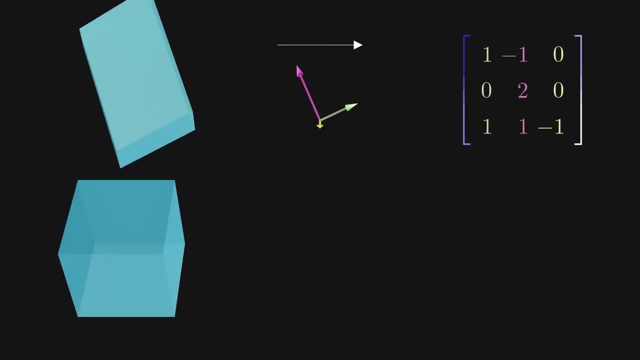 matrix representations. Earlier we said that the three columns of the transformation corresponded to where you sent the x, y and z unit vectors. Now let's take a look at the linear transformation of 3D space. We can see that the three columns of the transformation correspond to where you sent. 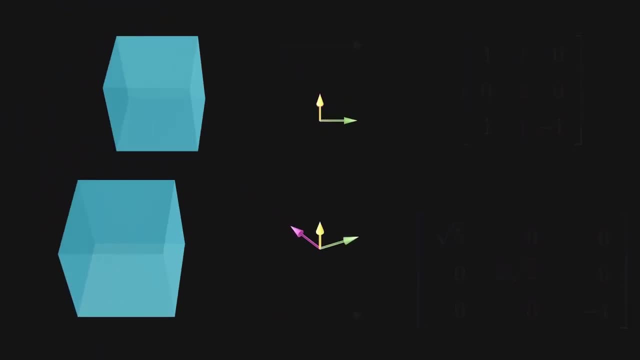 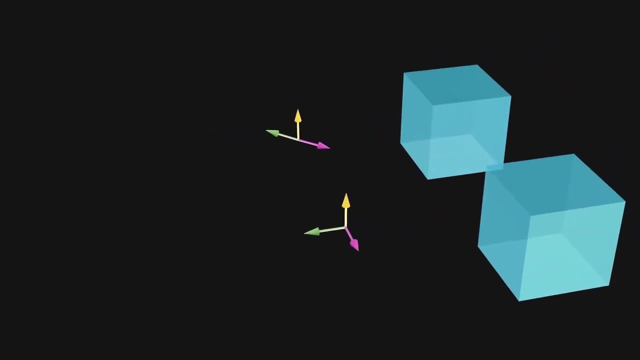 the x, y and z unit vectors. But the big idea of diagonalization is that you can instead describe where different basis vectors go. We can pick a set of basis vectors that are only scaled by our transformation, so that our representation is of a diagonal form, How we model 3D space in.